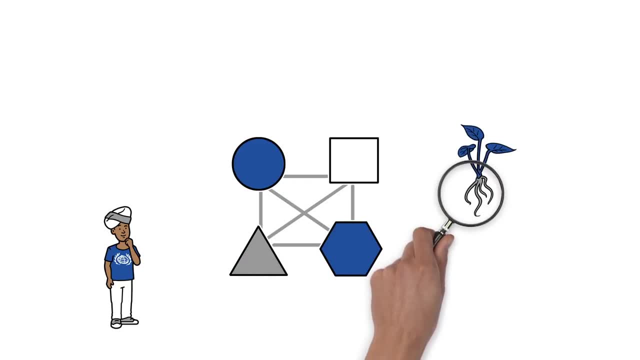 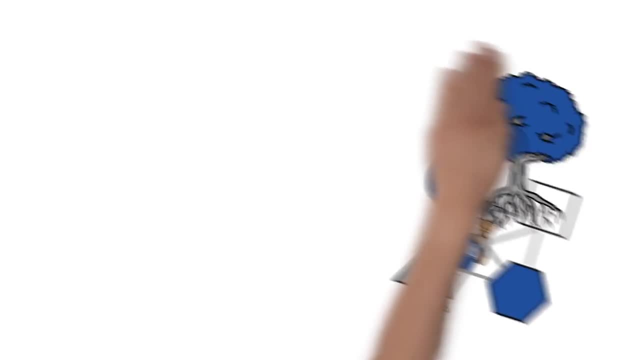 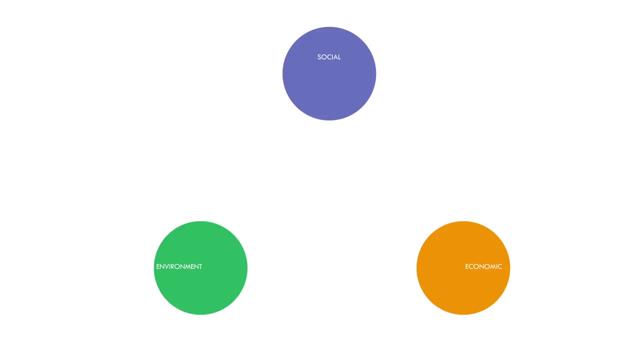 Finding these interdependencies helps us to address the root causes of problems and to create long term solutions. So how does this work? Sustainable development is usually viewed through a lens of three core elements: Economic growth, social inclusion and environmental protection. But it's important to remember that these are not just categories or boxes. 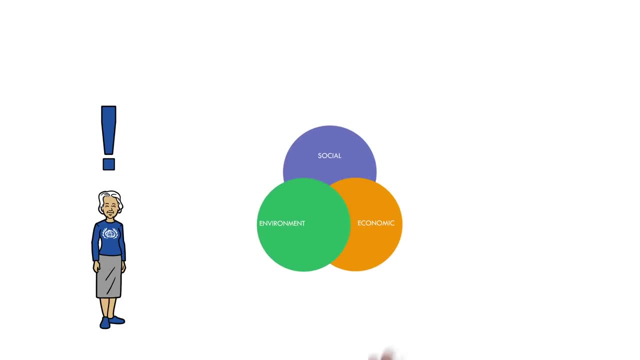 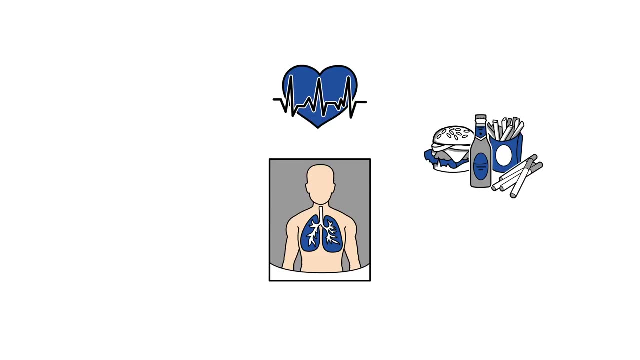 They are connected and have aspects in common. For example, a health challenge like tuberculosis is not only determined by an unhealthy lifestyle. It could also be influenced by other factors such as poverty or air quality. Agenda 2030 is an educational video. By endorsing Agenda 2030, we can. 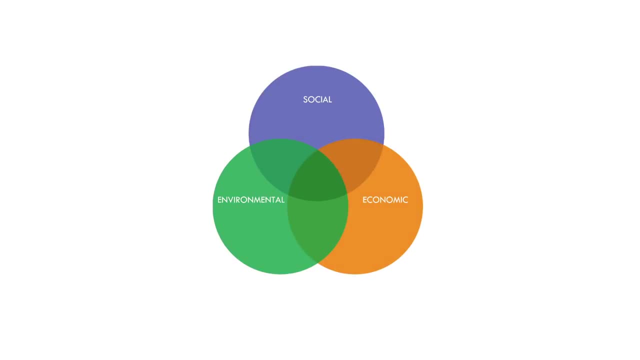 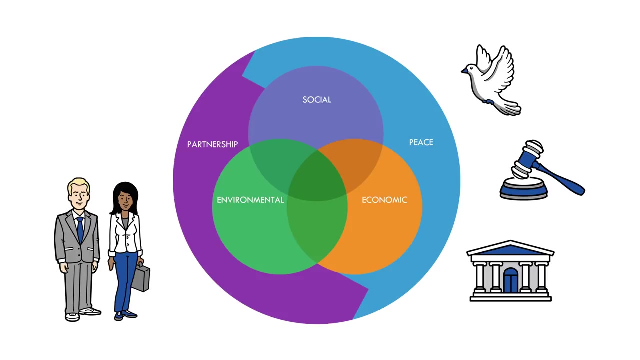 create a sustainable development for all countries. To develop this approach a step further, two critical dimensions that will drive Agenda 2030 were adopted by member states: Partnership and peace. Partnerships strengthen the capacities of all stakeholders to work together. Peace, justice and strong institutions are essential for improvements in the three core areas. 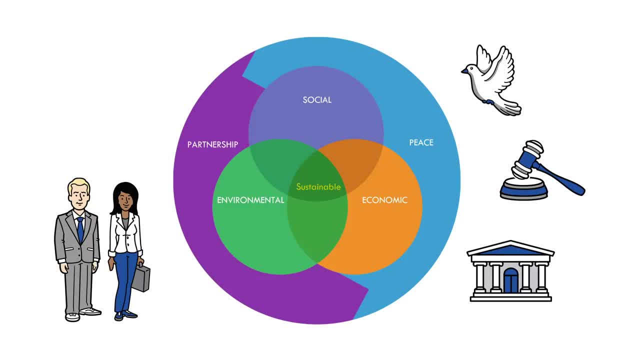 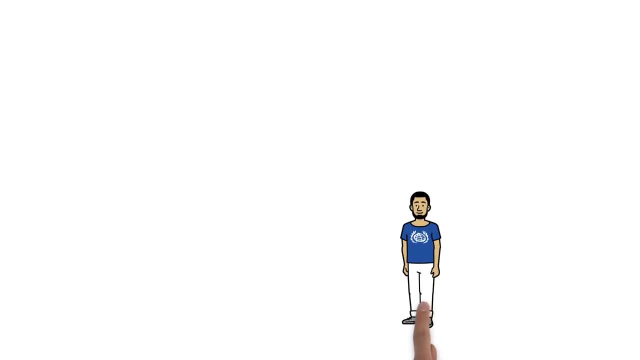 Genuine sustainability sits at the center, and it will be important to consider each of the SDGs through the lens of these five dimensions. Of course, we can't consider every possible angle of a single challenge. That's why it's crucial to build partnerships, to share knowledge and expertise, to learn how we can jointly address challenges. 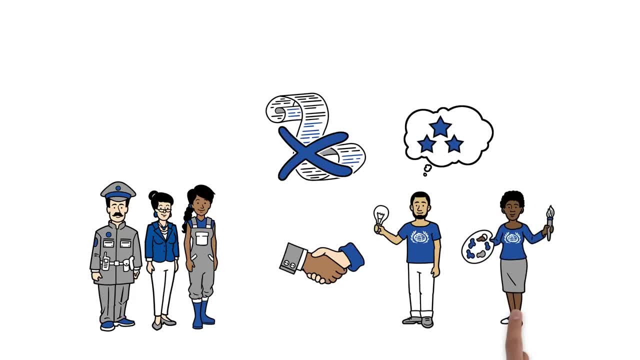 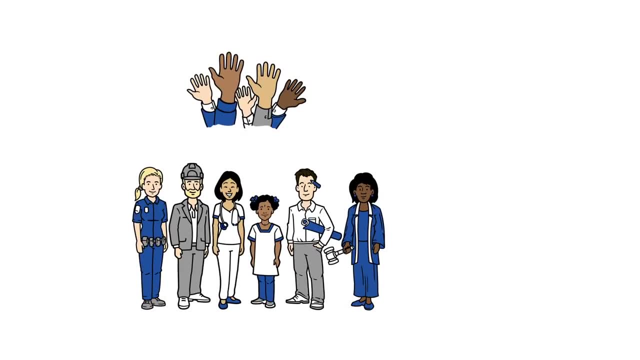 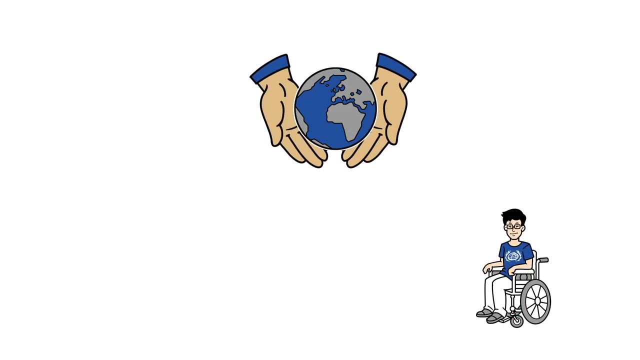 This requires new ways of working together, focused on co-creation. National ownership is fundamental to address challenges properly. Many organizations and actors have an important role to play. Their involvement ensures long-term engagement and guarantees that no one is left behind. The universal nature of Agenda 2030 also asks us to look at the planet as one. 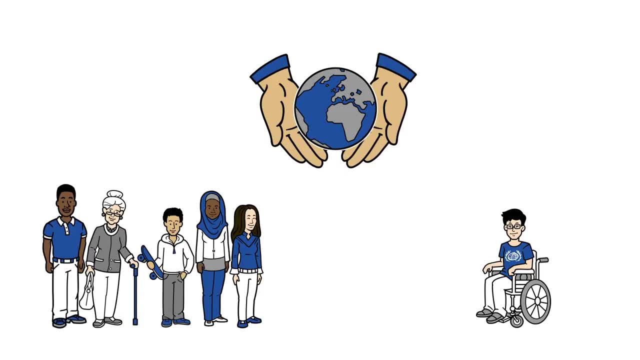 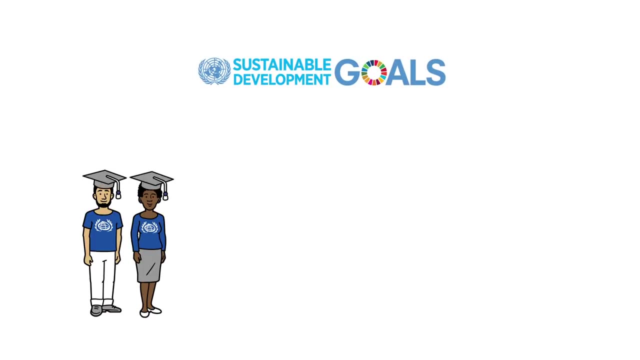 Every country, every community has issues to address and everyone shares the responsibility and ownership to address the challenges that face us collectively. To move forward, we must develop the right capacities for Agenda 2030.. We need to invest in lifelong learning to be able to advocate for change. 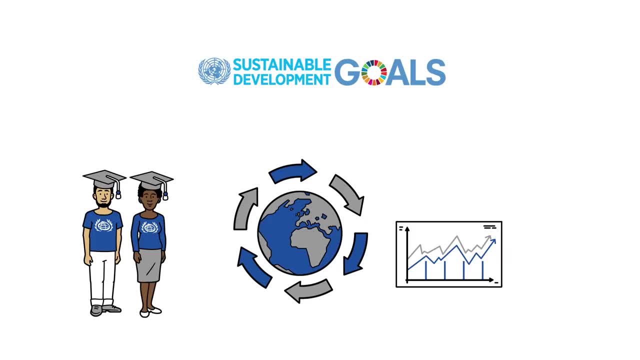 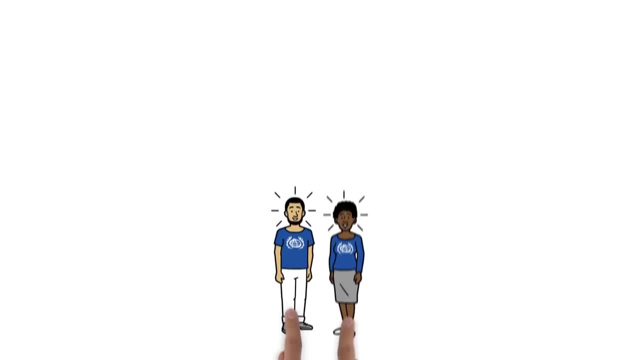 foster action for implementation, measure progress and to identify and empower new partners to support Agenda 2030.. We all need to lead the way towards the vision of a better world within our lifetime, Because only if we ask the right questions and seek the right answers.